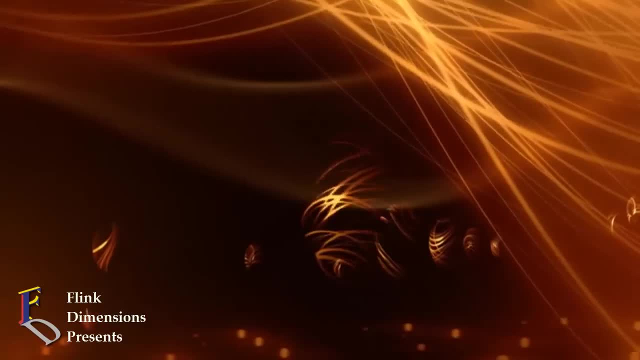 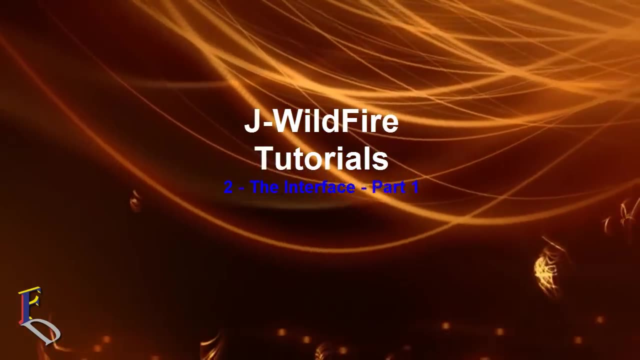 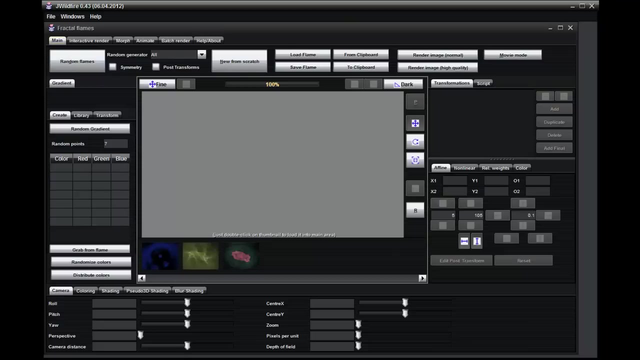 Hi there, Martin Flink here Just want to sort of kick off the second tutorial of JV Wildfire's amazing fractal design and graphics, as well as animation software, with a quick look at the interface. What we have here is, as you can see, a lot of buttons, a viewport and 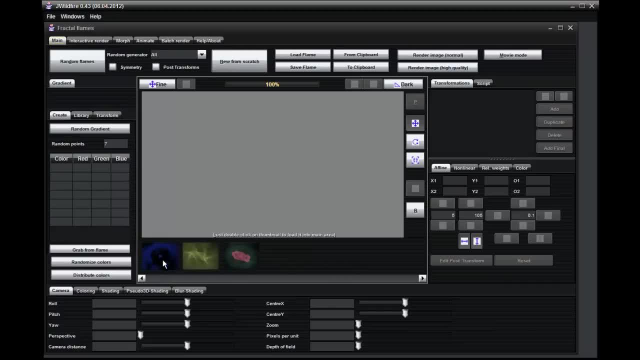 a couple of little thumbnails down here. These are thumbnails of the currently active or available flames inside of JV Wildfire. Now, the first thing I'm going to show you is a very simple little thing that a lot of people might not find otherwise, and that is, if you 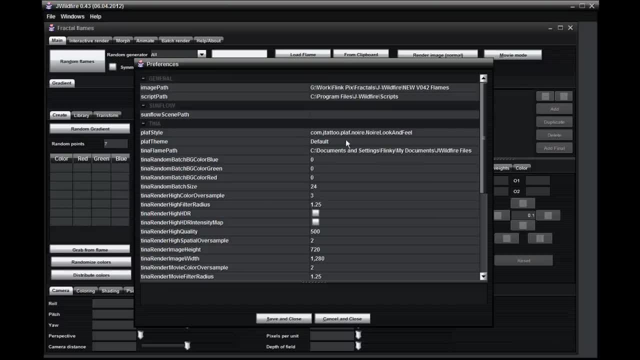 go to windows preference, you have all your image paths, scripts and all that kind of stuff if you want to get into that kind of level. But this is the one I was going to show you- that you can change the look and feel of the whole interface, and that's actually. 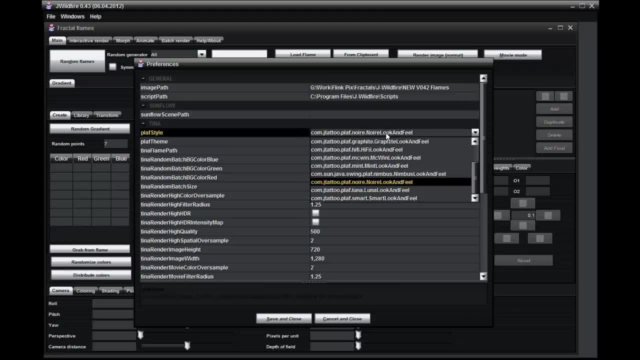 called PLAFF style. So what you do here is you go and double click on it and you get a whole list of different types here. Just try them, and you also have to restart the program and it's actually seen down here. So in other words, you go and pick one. that 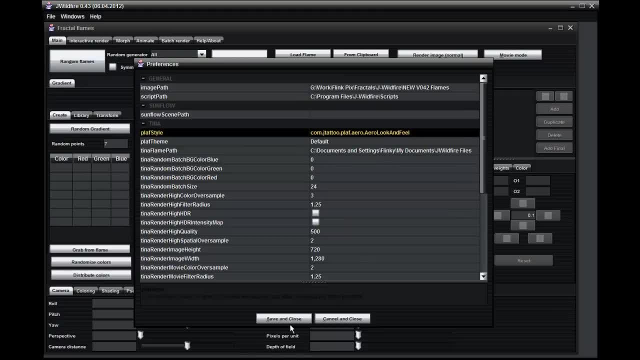 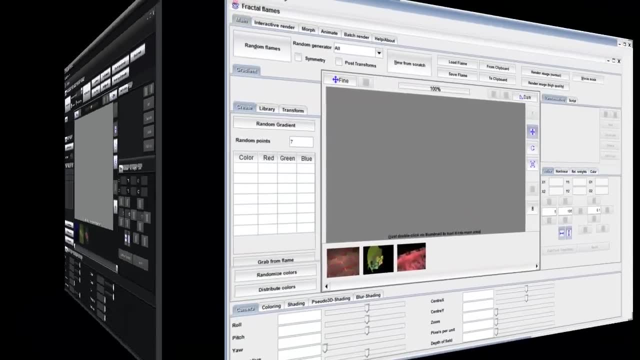 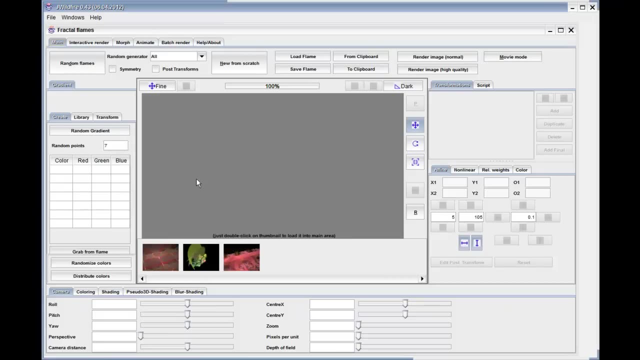 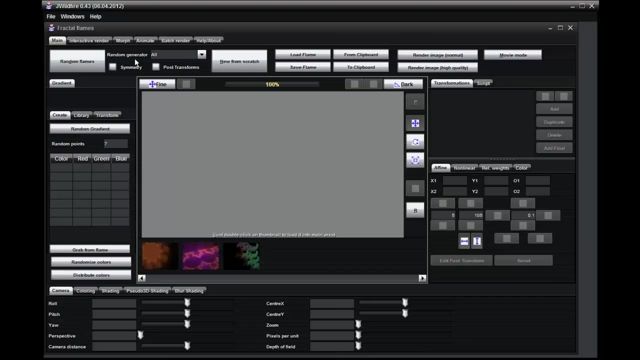 you like. So in my case, I'm going to pick the arrow look and feel, save and close the preferences, and then I'm going to just quit. And here we are back again. Now, this is the arrow version: look and feel, and nice and clean. Okay, so here we are. I decided to. 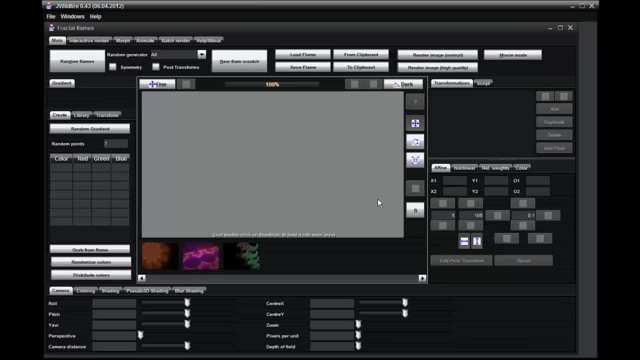 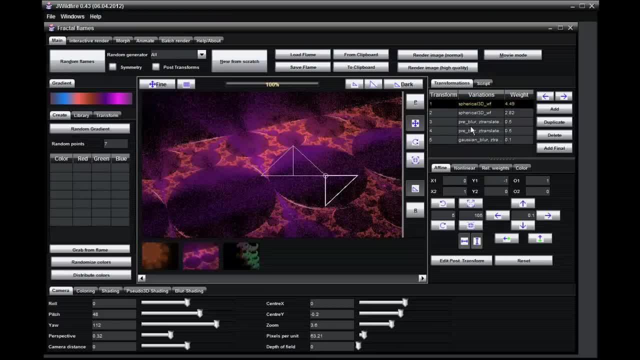 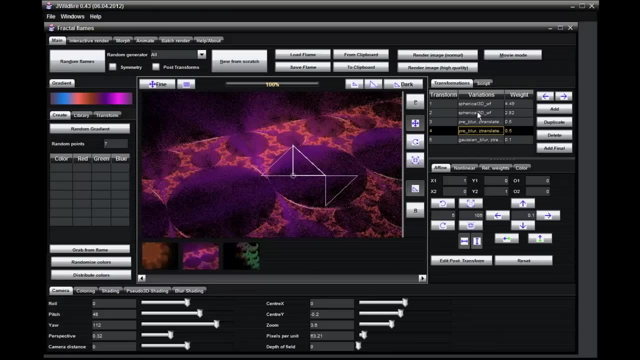 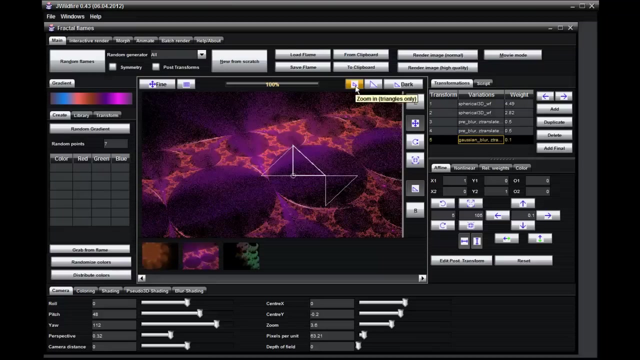 back to the standard interface. I kind of like it that way. So what do we do to get? We have a number of control buttons down here, like Fine, to display and hide variation effects. I'll do that when we start on refresh with a new transform. 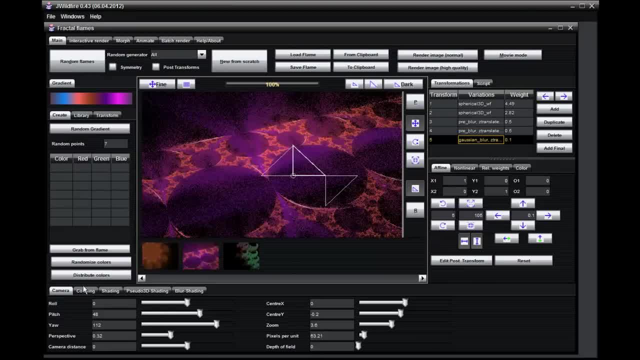 Zoom in and out to do with the triangles display Down here we have the camera, all the camera settings. in the bottom here We have coloring, shading, pseudo 3D shading, blur shading. A couple of buttons down here and this one here is to sort of toggle the post transform. 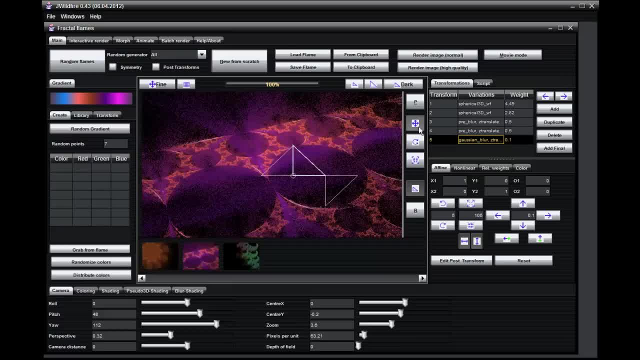 mode and enable triangle dragging mode, which is by default, is switched on, So we can actually basically just go in and anywhere on the viewport. you don't actually have to drag the. you know you don't have to be very accurate here, just anywhere, because 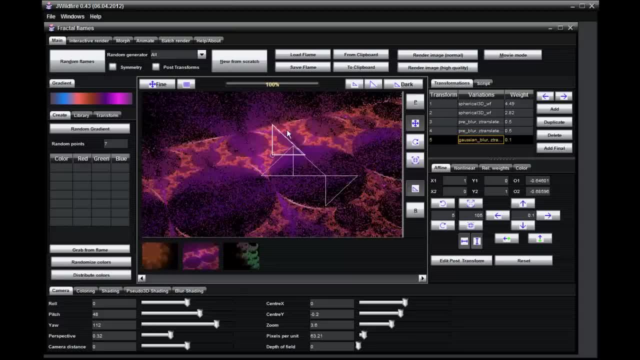 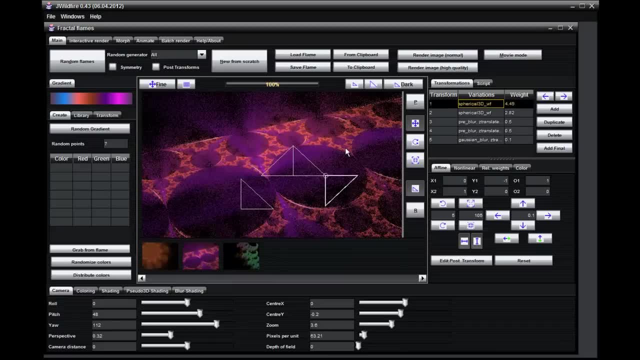 the selected one is the one that's going to shift. So I'm starting here just to move that triangle, and I can see what's going on in here in the viewport. Let's take something that does a little bit more. So I'm just going to take that one there and start dragging it around a little bit. 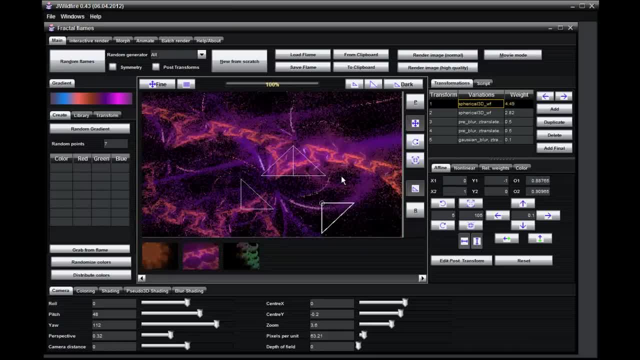 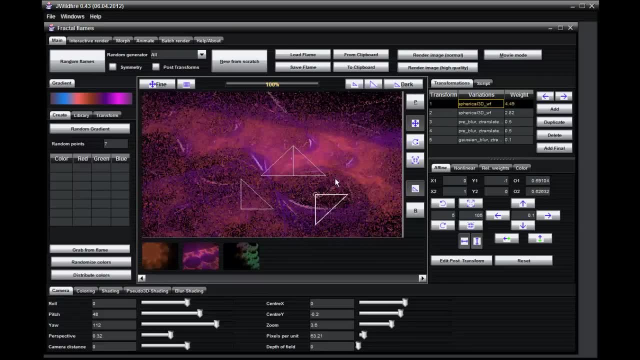 And, as you can see, little shifts could kind of completely change the result. Okay, If you're doing a bit of messing about and you want to be sure that you can get back to your initial setting, the best way to do that is to use the other interface for moving. 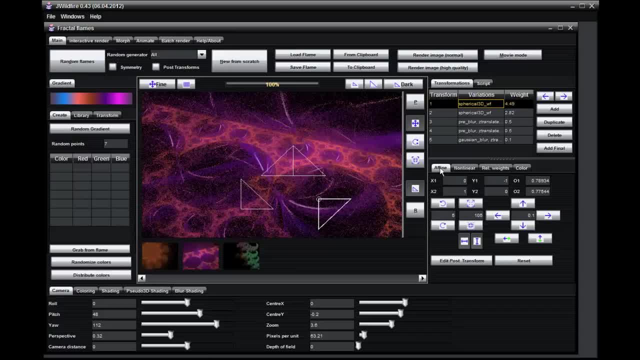 and scaling and so on. And that's over here on the right. the affine tab, The affine transformations are to do with your actual triangle that you've selected, And here you can set the actual moves, for example, or you can type in your actual you. 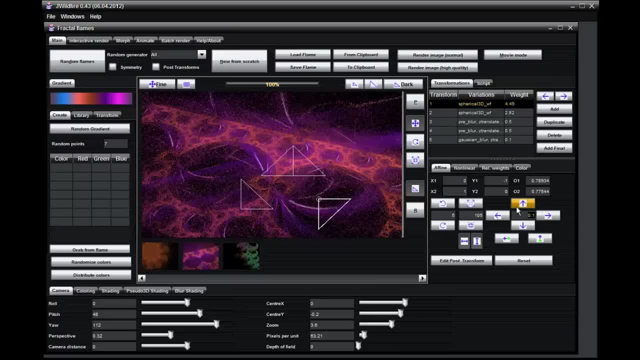 know coordinates here: X1,, X2, and so on. Your buttons here allows you then to move the triangle in little increments or in big increments. So if you want to check something out, you might want to put in a reasonably large number. 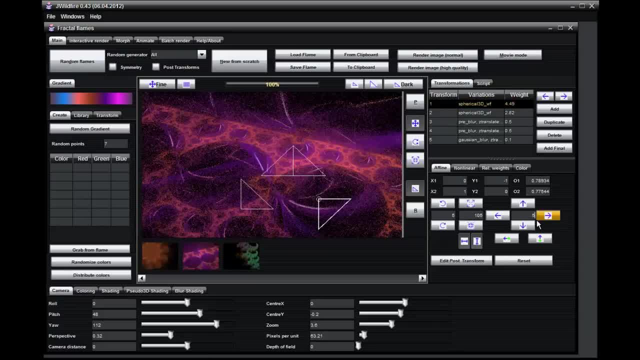 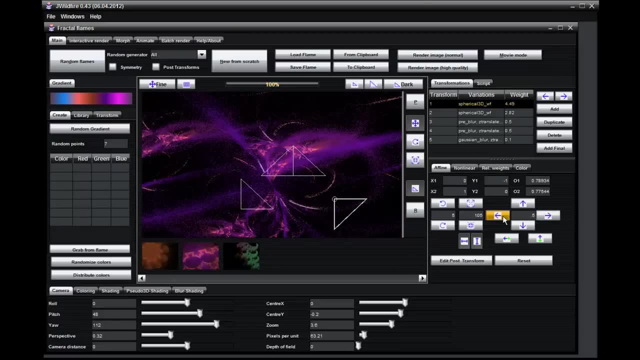 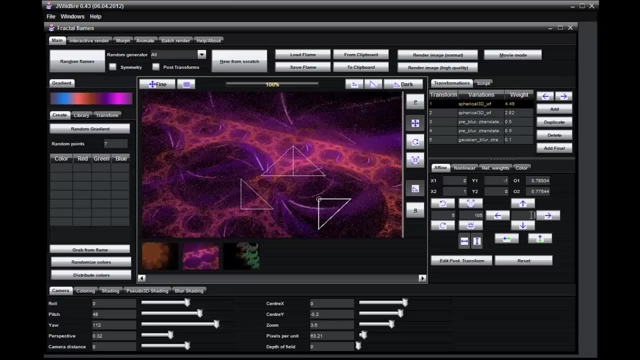 like 0.5, you need to basically hit enter or carry return in order to get it to take anything you type in. All right, Now this one is fairly sensitive, so we're just going to take that down to zero point and put in the leading zeros one, to just kind of make it look neater. 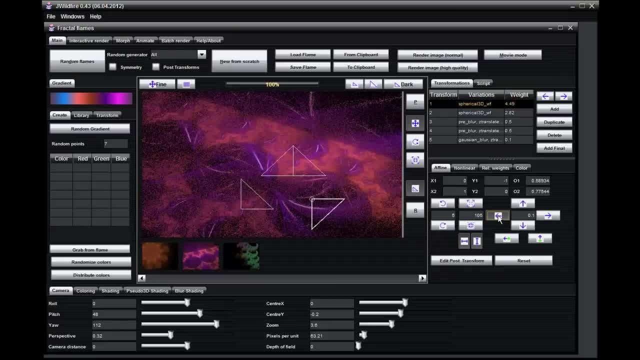 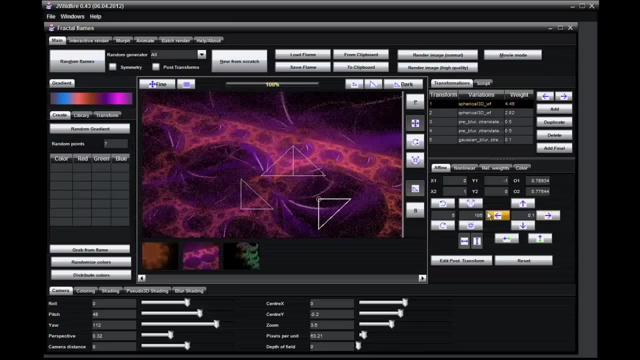 And now we can see it because it's not quite as wild. So I just, you know, and if I wanted to go back, all I have to do is just go back, because now we're doing a defined step here, So it's much easier to kind of make sure you come back to where you started. 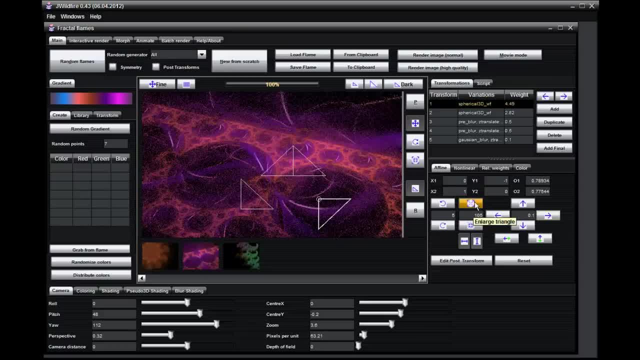 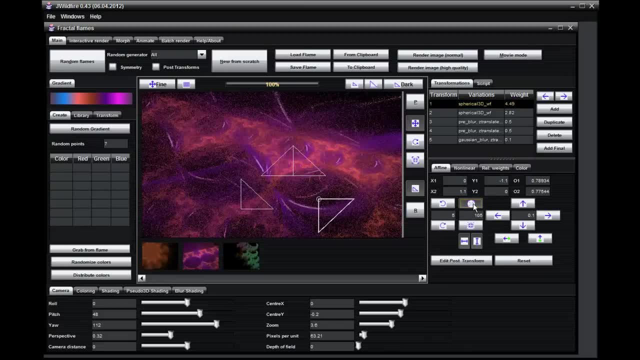 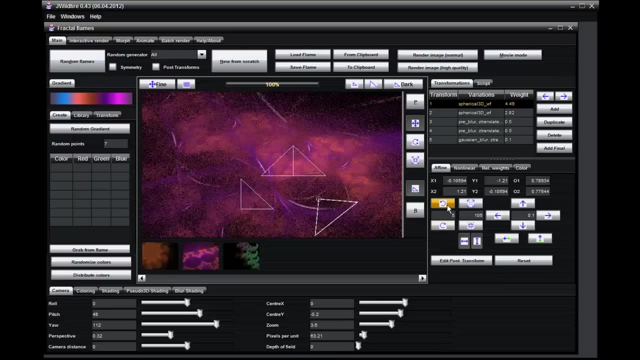 Assuming- to enlarge the triangle or shrinking it, you can just go in here and use those ones. So I'm going to give it five percent each time so you can kind of enlarge it like that. Or you can rotate them by five in this, in this case five degrees, right? 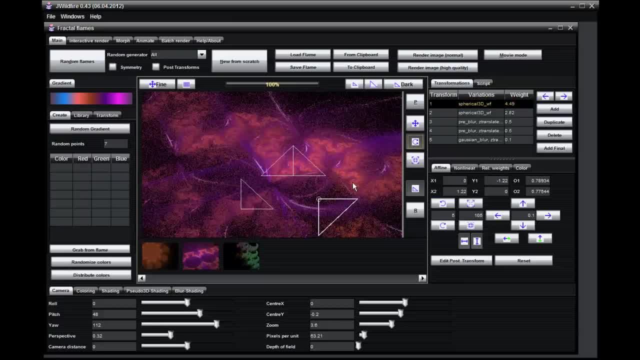 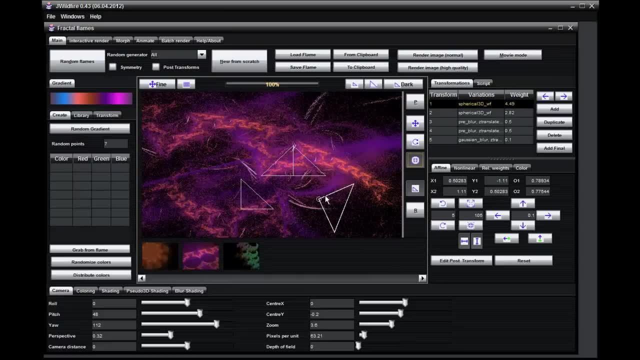 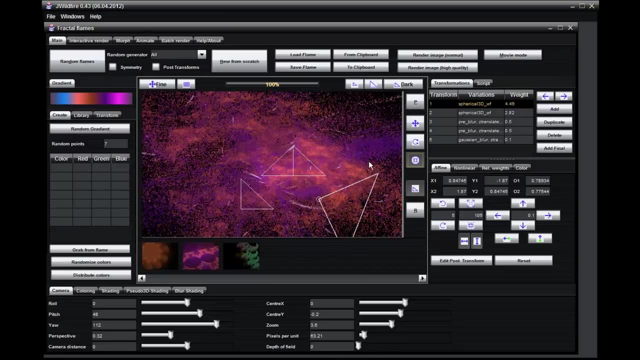 All these things you can do in here as well, So like, for example, rotate mode, shrink and scale mode. You can also do that by just grabbing the actual triangle, like this, but you don't actually have to. That's the cute thing about this. 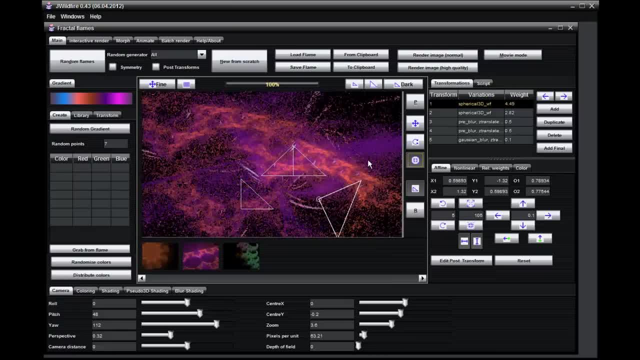 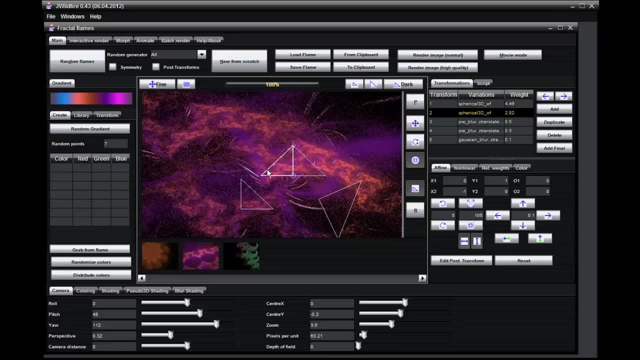 There's also shortcuts you can use on the keyboard for all these type of things- move and so on. Now, so you can also select by clicking on one. So if we want to get that one moving, we can just go in and click and drag on it. 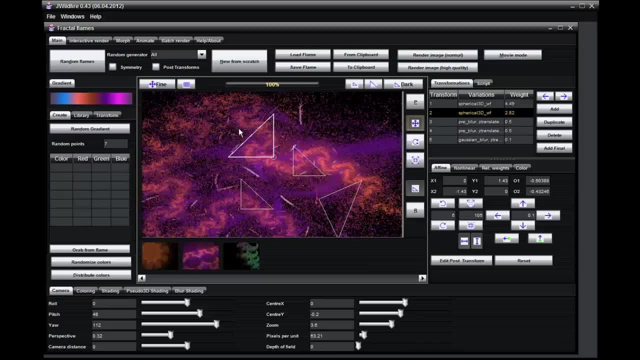 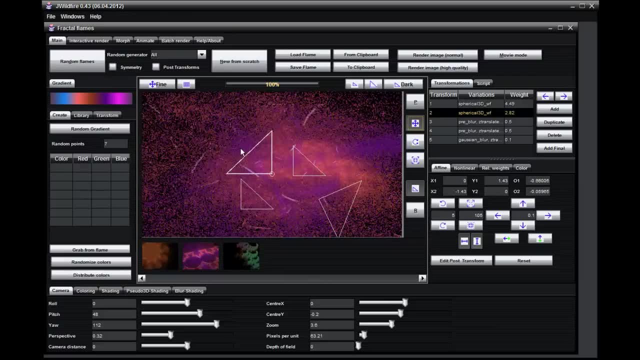 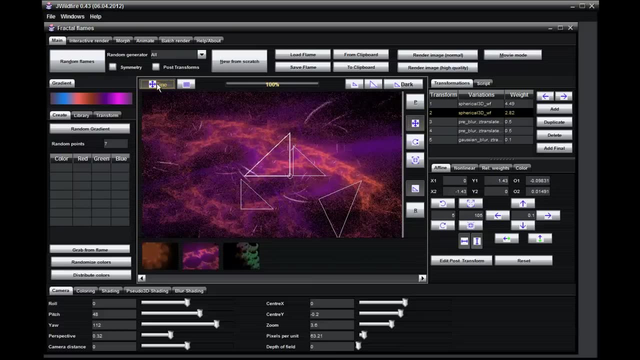 Now I'm going to move it again, get back to move mode and shift it around a bit, that particular one Now, as you can see, because we're dealing with chaos here and fractals. you know, slide it, The slide transformations is normally all you want. so therefore, if you click on, fine. 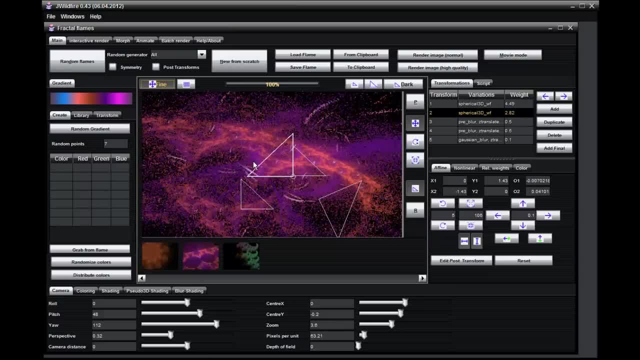 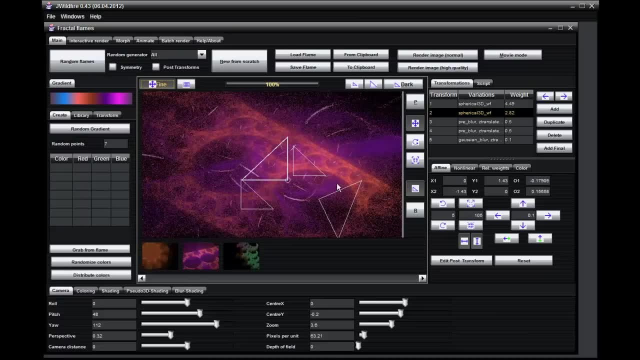 mode. it slows your mouse movements down a bit so that you can kind of, you know, drag fairly heavily. Now, when you got a result that you're interested in, you might want to either double click in the viewport or click on this button here: render image. 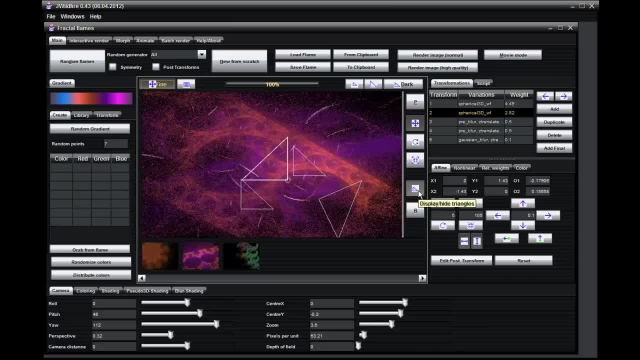 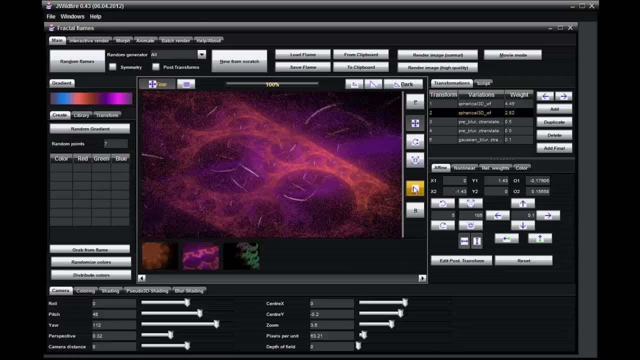 That would just renders to the viewport. so it's kind of a, you know, intermediate kind of slightly better render, And if you want to, If you want to have a nice clean view of it, you might just click on that to turn off the. 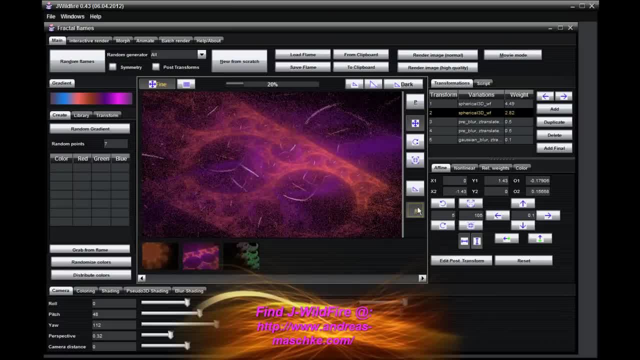 triangles view and then you see better what's going on.